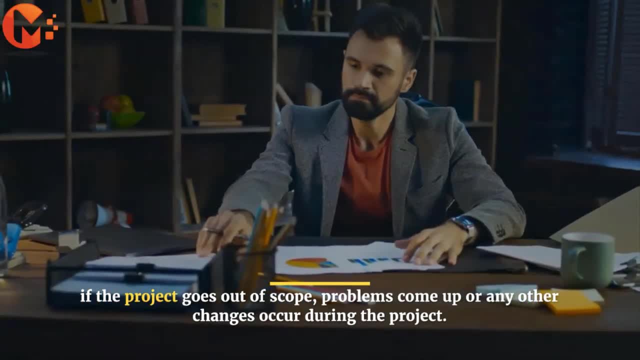 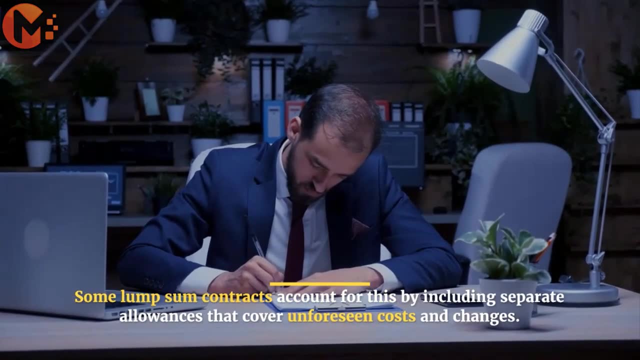 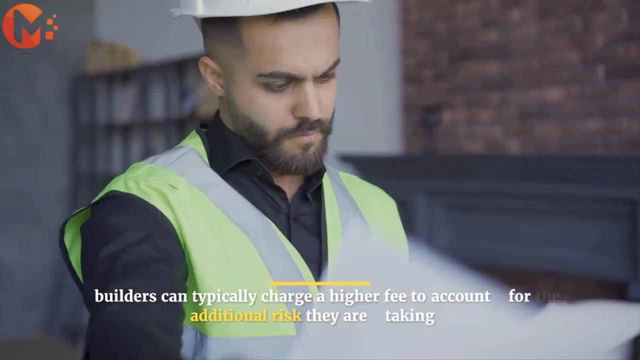 or any other changes occur during the project. Some lumpsum contracts account for this by including separate allowances that cover unforeseen costs and changes. If an owner decides to use a lumpsum contract on a project, builders can typically charge a higher fee to account for the additional risk they are taking on. Otherwise, any unforeseen costs can either eat into a builder's profit or result in a project that may not be completed as envisioned. Pros of Lumpsum Contracts: Builders have a clear expectation of the scope. Owners avoid paying unexpected project costs. Cons of Lumpsum Contracts: 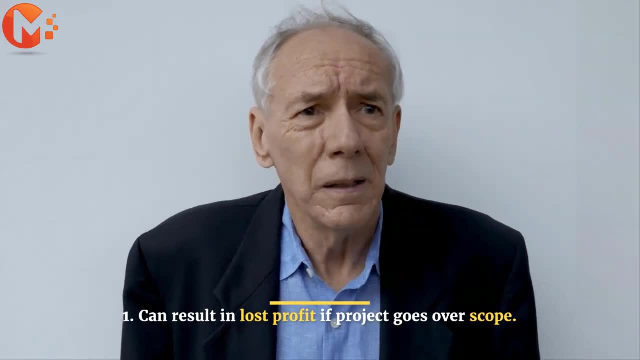 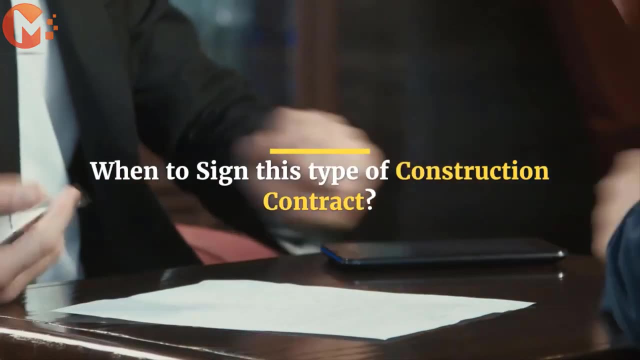 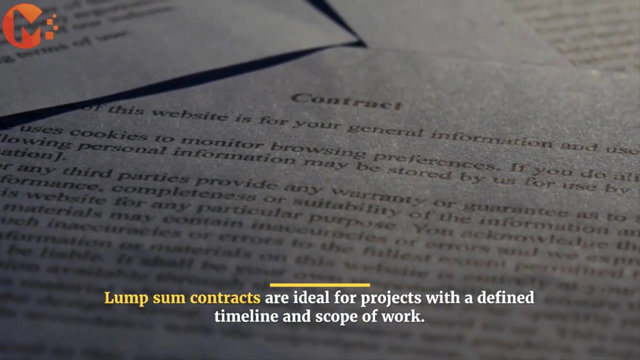 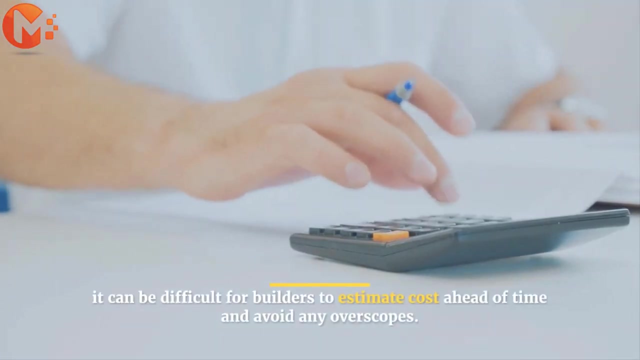 It can result in lost profit if project goes over scope. Budget constraints may limit project outcomes. So when to sign this type of construction contract? Lumpsum contracts are ideal for projects with a defined timeline and scope of work. If these are not clearly agreed upon, it can be difficult for builders to estimate cost ahead. 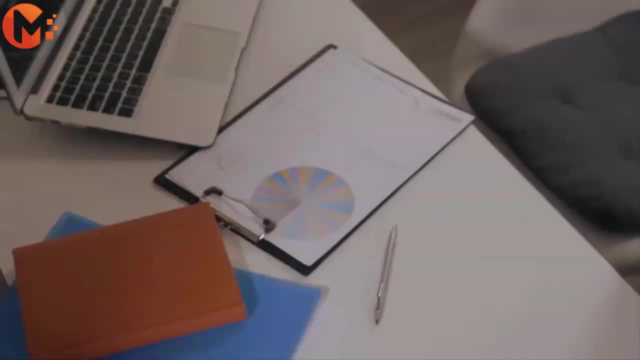 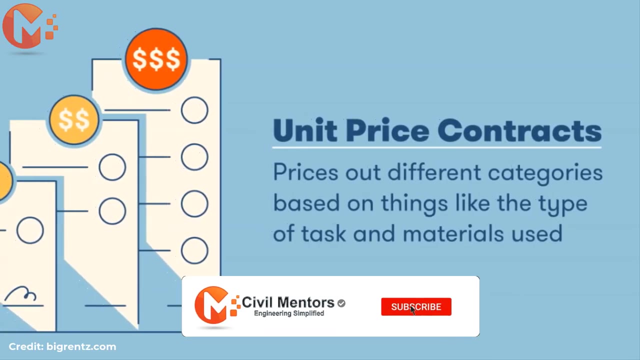 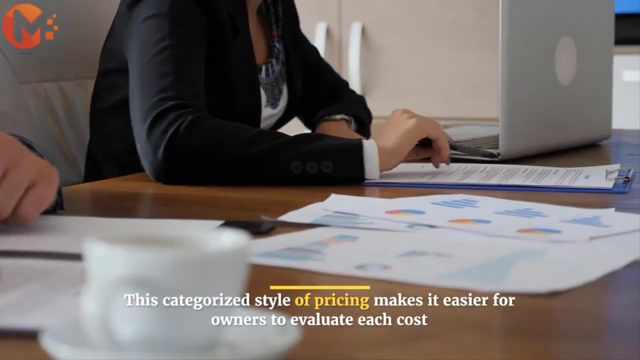 of time and avoid any overscopes. 2. Unit Price Contract. Unit price contracts typically emphasize the types of tasks being carried out, in addition to the materials used on those tasks. This categorized style of price contract is the type of makes it easier for owners to evaluate each cost and allows builders to more accurately. 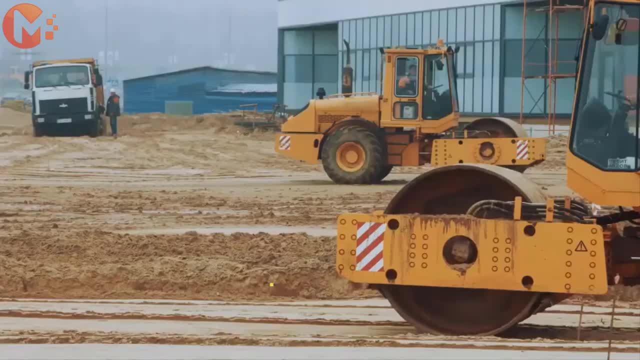 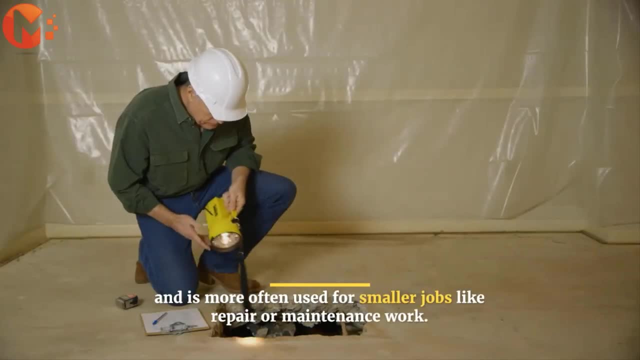 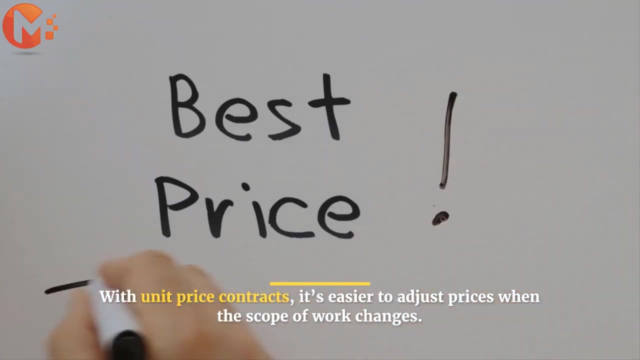 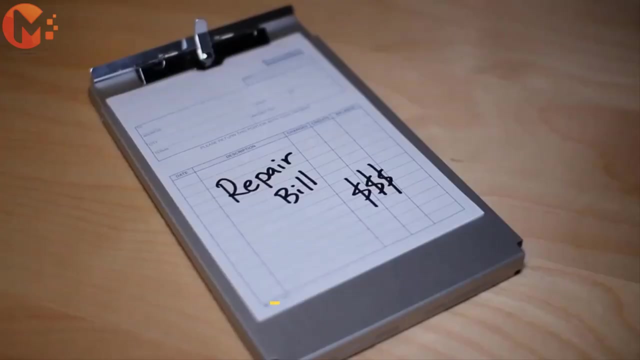 charge for each category. This type of construction contract is not typically used for major construction projects and is more often used for smaller jobs like repair or maintenance work. With unit price contracts, it's easier to adjust prices when the scope of work changes. Pros of unit price contracts: It is easy to evaluate costs of different categories. 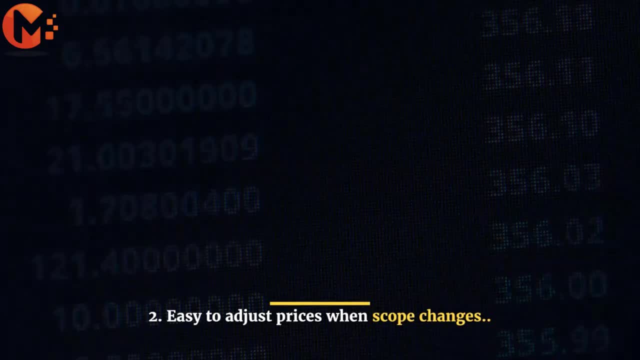 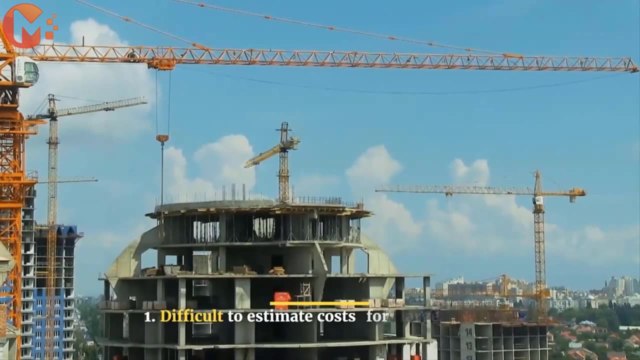 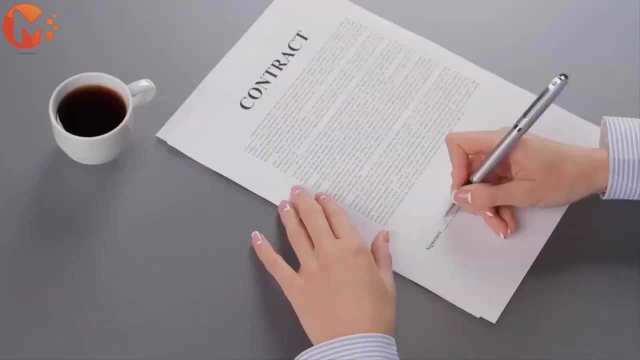 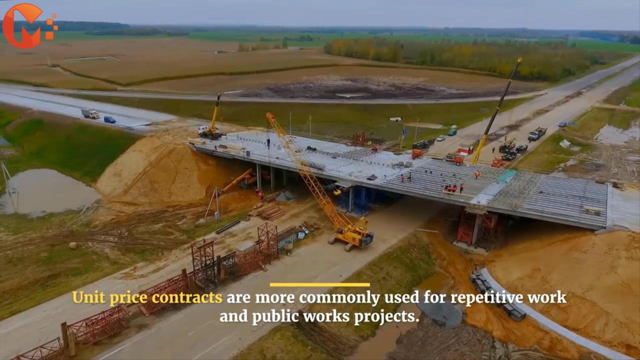 and also easy to adjust prices when scope changes. Cons of unit price contracts: Difficult to estimate costs. for large projects, Final cost is not defined in the beginning. So when to sign this type of construction contract? Unit price contracts are more commonly used for repetitive work and public works projects. For example, routine building maintenance could more easily be charged through a unit price contract, since it specifies the values of different maintenance tasks required. Number 3. Cost plus contract. Cost plus contracts normally require the owner to pay for all project expenses, like the cost of materials, labor and any other. 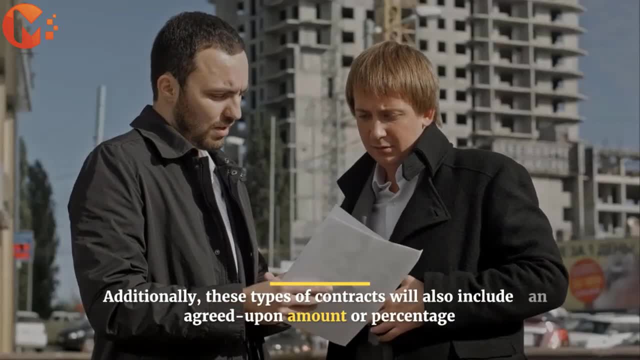 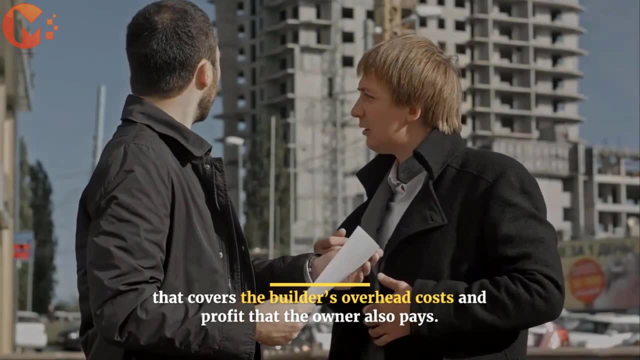 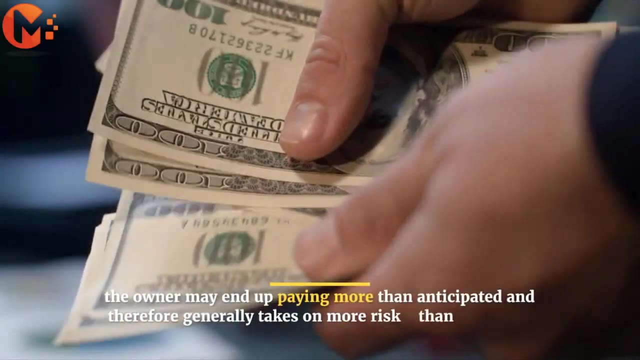 projects costs. Additionally, these types of contracts will also include an agreed-upon amount or percentage that covers the builder's overhead costs and profit that the owner also pays. Depending on the type of cost plus contract, the owner may end up paying more than anticipated and therefore generally takes on more risk than the builder. 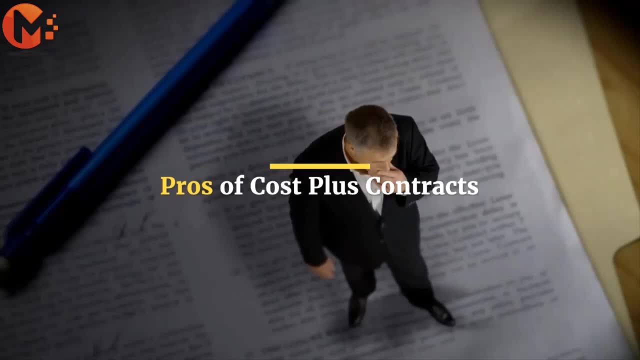 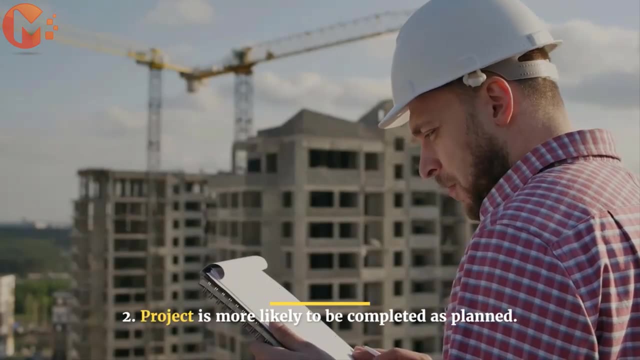 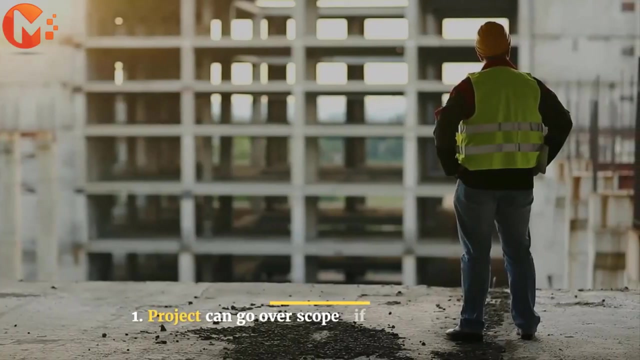 Pros of cost plus contracts. Pros of cost plus contracts: It reduces risk for builders. Project is more likely to be completed as planned. Cons of cost plus contracts: Project can go over scope if caps are not applied And it is difficult to manage and track. 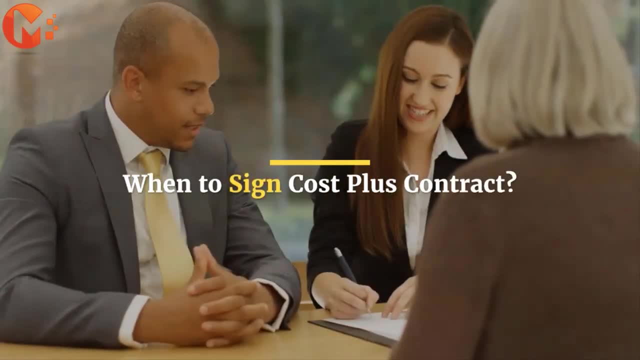 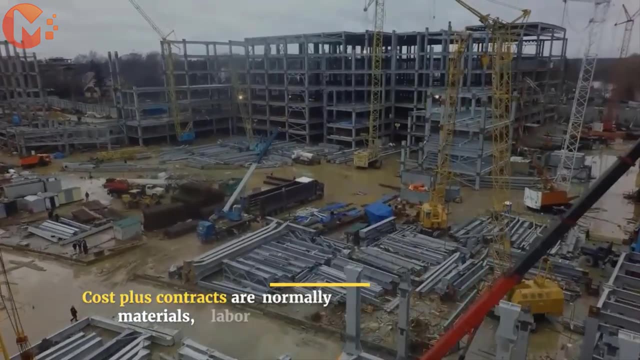 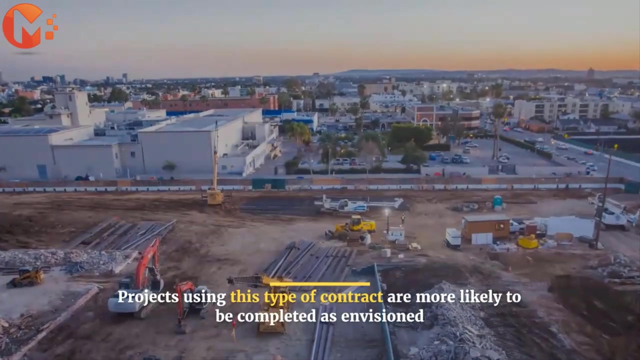 So when to sign cost plus contract? Cost plus contracts are normally used when the scope of work, materials, labor and equipment are not clear, itan equivalent or not clearly defined or difficult to estimate from the beginning. Projects using this type of contract are more likely to be completed as envisioned. 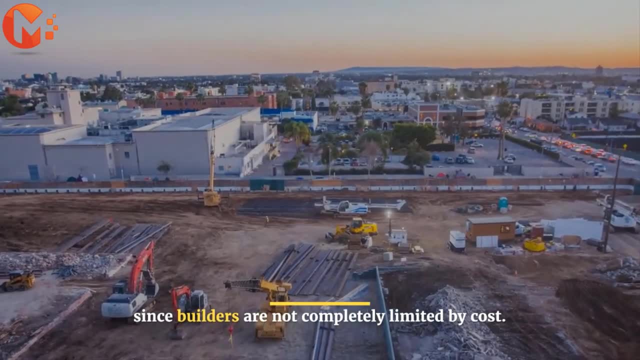 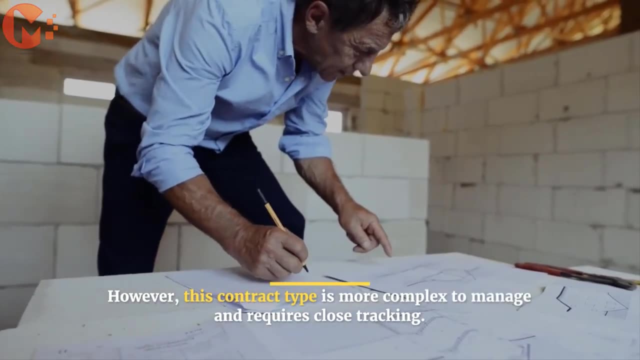 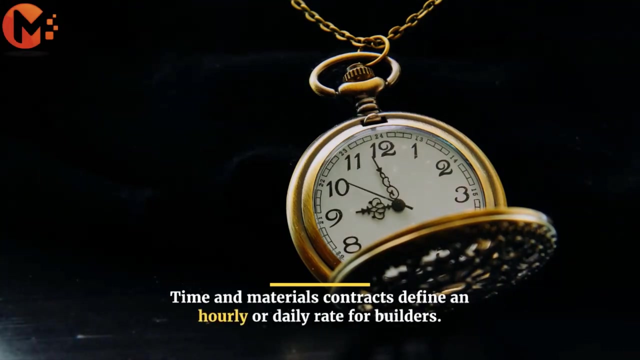 since builders are not completely limited by cost. However, this contract type is more complex to manage and requires close tracking. Number 4. Time and materials contract. Time and materials contracts define an hourly or daily rate. Time and materials contracts define an hourly or daily rate. 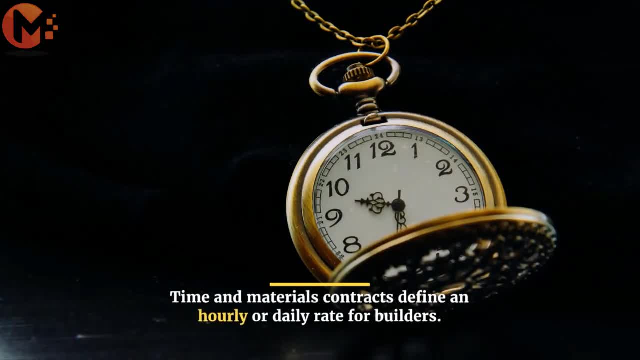 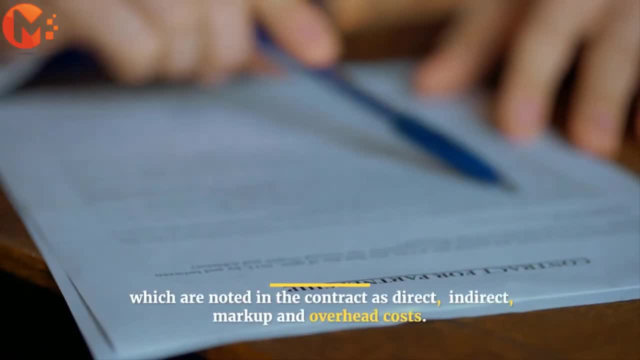 It is well known that most buildings of this type are classified as long-term contracts or daily rate for builders. In addition to paying this rate, owners also agree to pay any related project costs which are noted in the contract as direct, indirect markup and overhead. 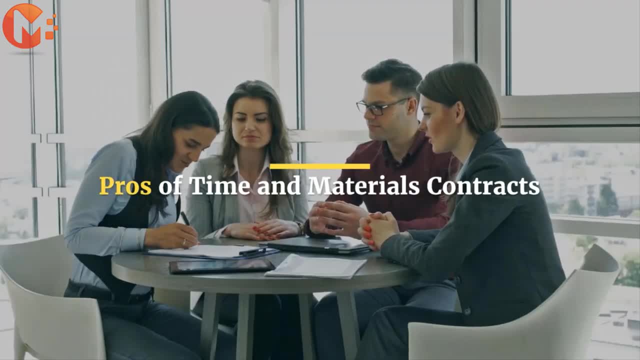 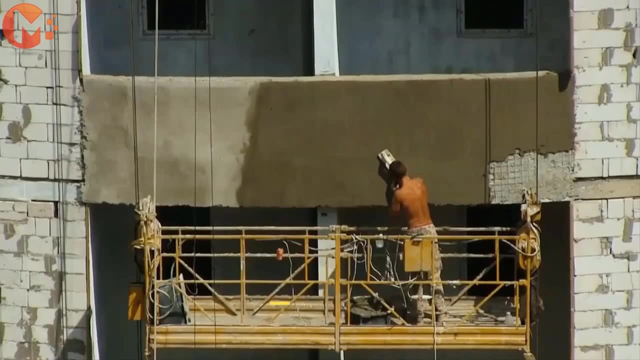 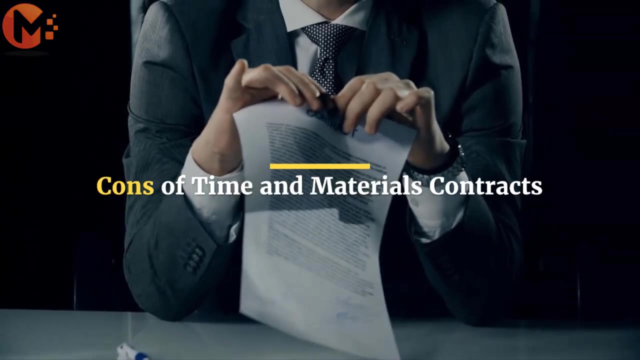 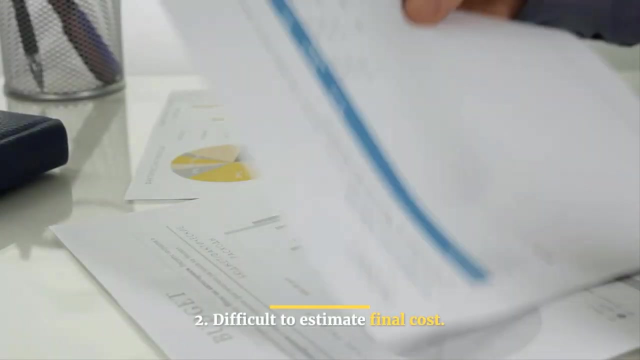 costs. Pros of time and materials contracts. Builders are not completely limited by budget. It is easy to use for small projects Cons of time and materials contracts. Project can go over scope if caps are not applied. Difficult to estimate final cost. 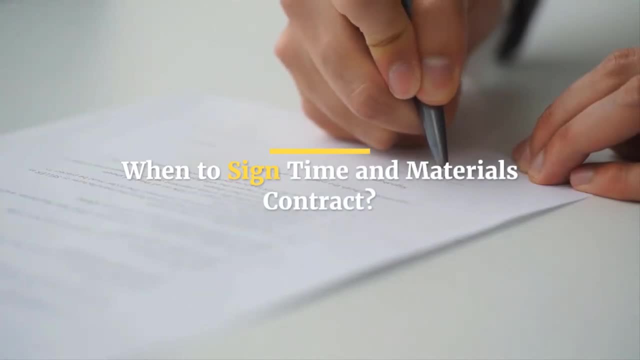 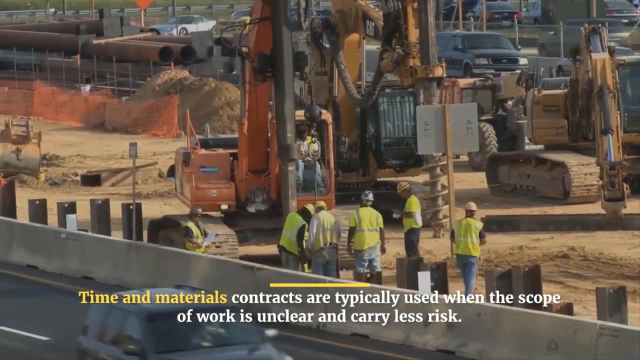 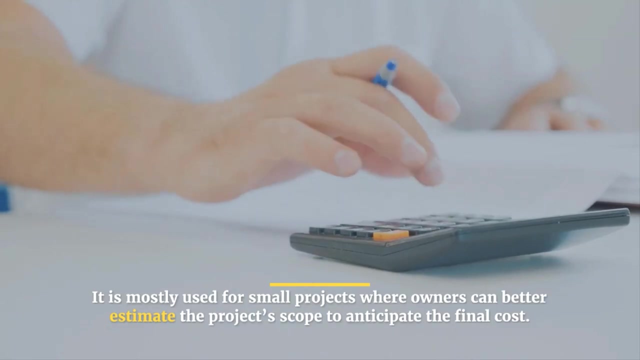 So when to sign time and materials contract? Time and materials contracts are typically used when the scope of work is unclear and carry less risk. It is mostly used for small projects where owners can better estimate the project's scope to anticipate the final cost. 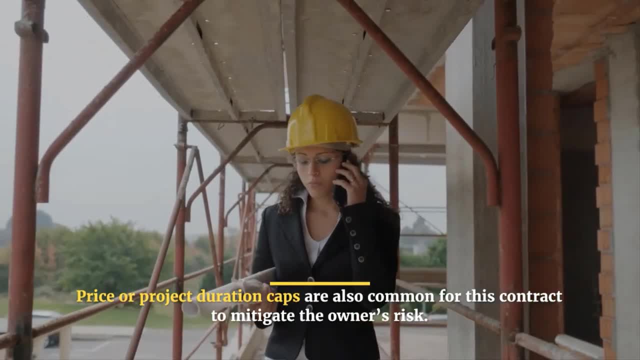 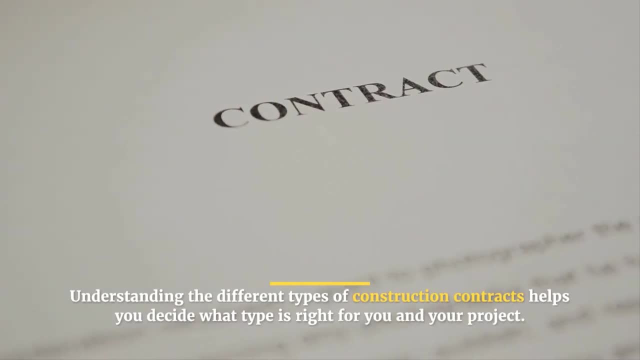 Price or price of work. Price or price of work- Project duration caps are also common for this contract to mitigate the owner's risk. Understanding the different types of construction contracts helps you decide what type is right for you and your project. Along with the contract, there are many other. 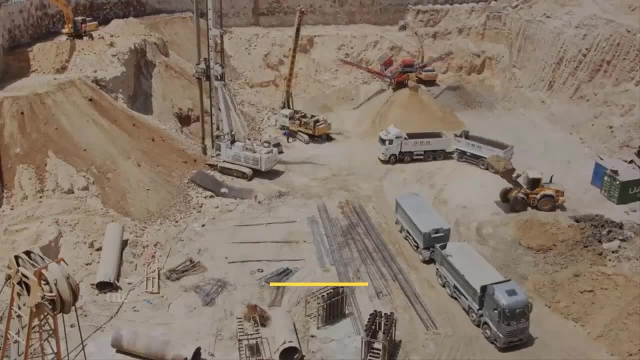 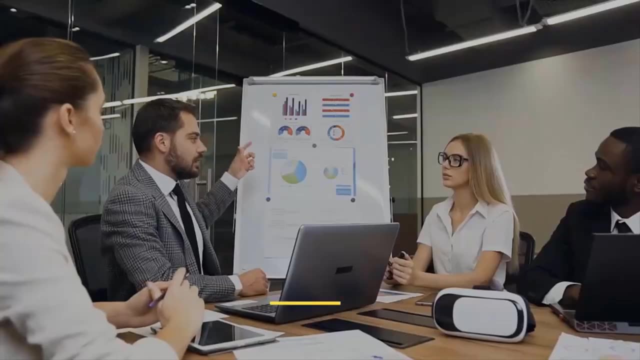 moving parts to consider, like the amount of labor you will need, the construction technology you should consider and the major machinery you will need for the job. Also, consider implementing value engineering into your next project to help you understand the different types of construction contracts.